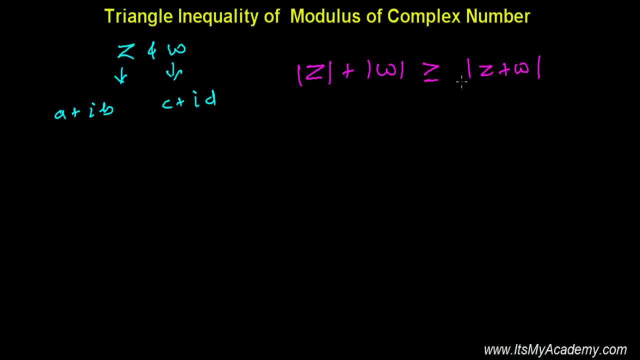 The sum of those complex number. right, Let me tell you once again: the individual sum of the absolute value of the two complex number is always greater than or equals to the absolute value of the sum of those two complex number. all right, So let's examine how it is, whether it is true or not. okay? So here we have z. absolute value of z, that is a square plus b square under root, and absolute value of w is c square plus d square. 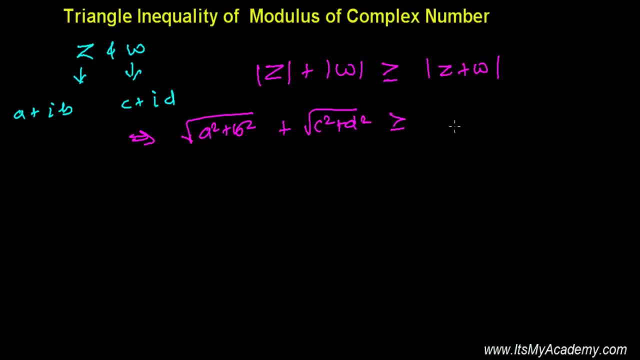 All right, and is greater than or equals to z plus w. z plus w, if you do, you'll get a plus c, and plus i times b plus d, you'll get all right, and we need to find out the absolute value of that. it's absolute value of z. all right, it's very bad, I'm sorry. it's a square plus b, square inside the root, plus c square plus d, square inside the root is greater than or equals to now: a plus c whole square, plus b plus d, whole square. 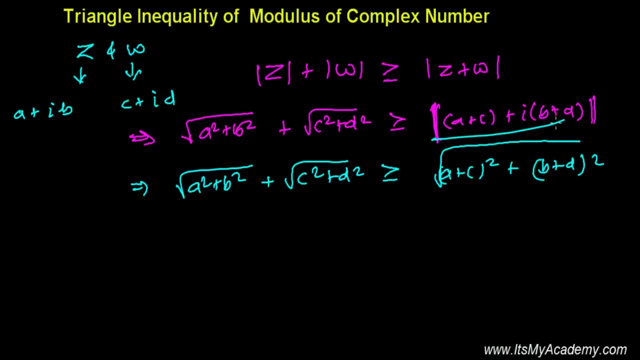 All right, we find out the actual value of this complex number also. Now let's square both side. if we square both side, we can apply here a plus b whole square formula. so it will be a square plus 2 a, b plus b square, right, that's d square and is equals to or less than or equals to 2 a, b plus b square. 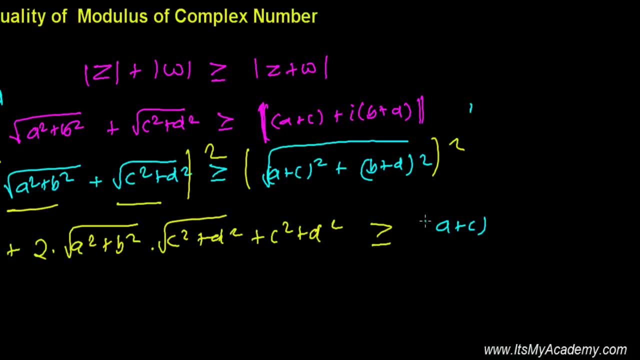 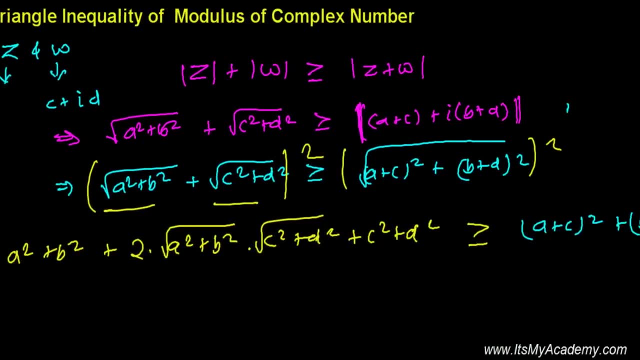 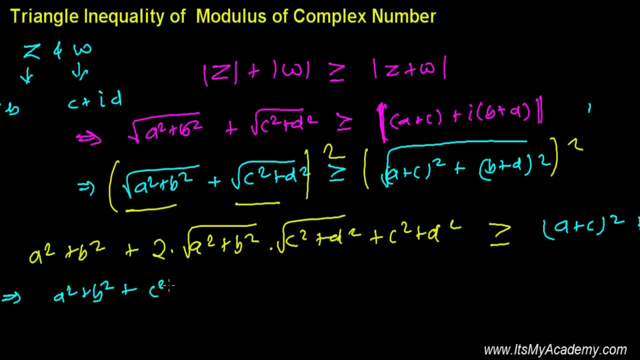 Again this one that is simply a plus c whole square plus b plus d whole square. now, root has been removed from left hand side, right hand side also. so I think further. we need to write this: a square plus b square. let me write this: c square plus d square and now 2: a square plus b square inside the root. c square plus d square inside the root is greater than or equals to a plus c, b plus d square. 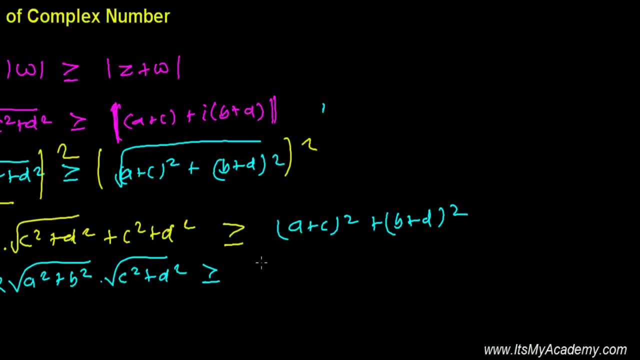 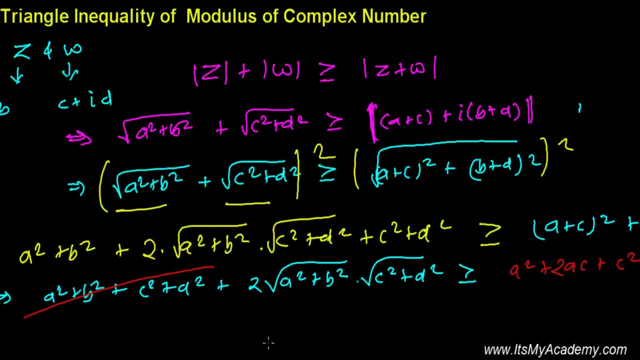 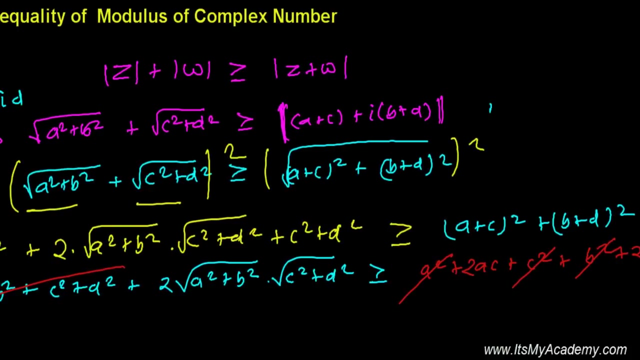 So again, let's apply the formula of a plus b, a plus c whole square. so it will be a square plus 2, a, c plus c square, and here also b square plus 2, b, d plus d square. So now look at here, few thing is being cancelled: a square, b square, c square, d square. this all four and a square, c square, b square, d square will cancel up. and now we'll get here next thing: after cancelling, you'll get this 2, okay, let's first take common right. 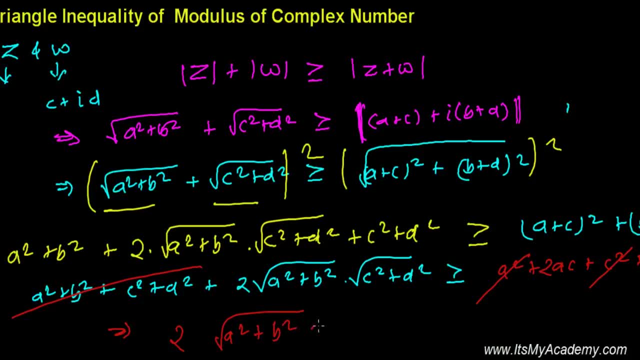 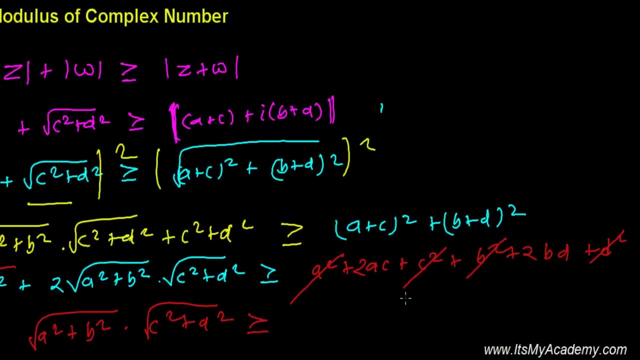 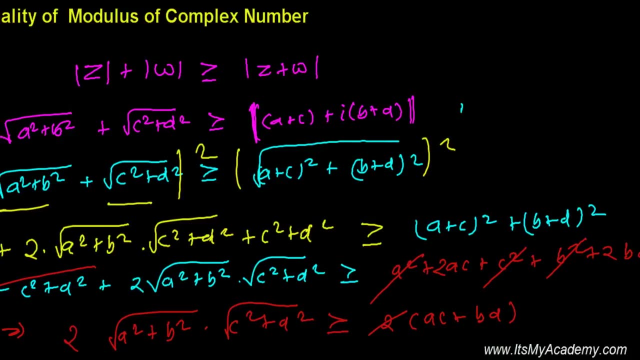 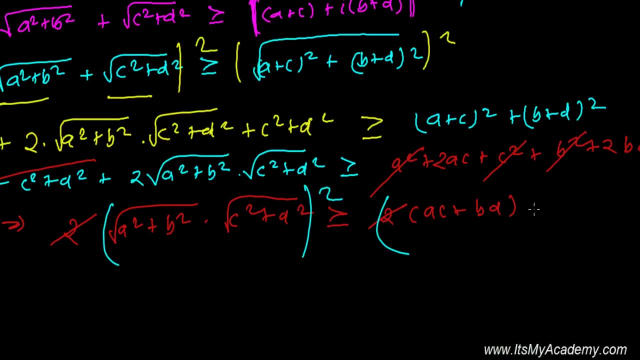 2, a square plus b square. inside the root c square plus d square is greater than or equals to 2 b d, 2 a c. so I'm taking 2 common and it will be a c plus b d, alright. And this 2, and this 2 will cancel up and after cancelling the 2, what I'm doing, I'm going to square both side now. I square here, I square here, so it will be now a square plus b square times. 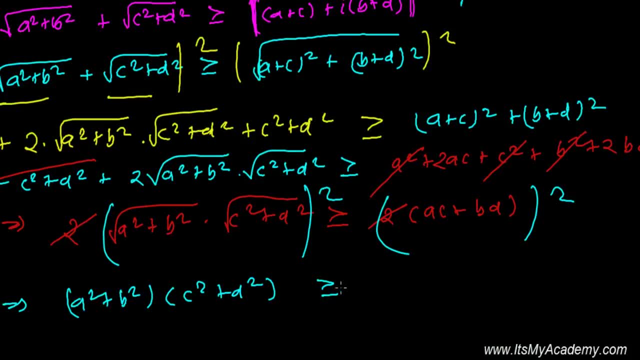 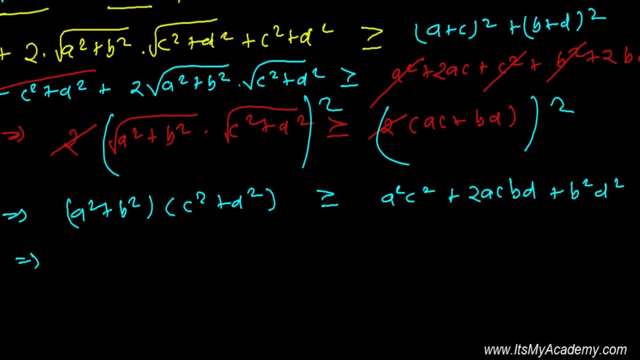 c square plus d square is greater than or equals to. squaring this, it will be a square c square plus 2, a, c, b, d plus b square d square. alright, And so now let's multiply this. a square will be plus c square, so it will be a square c square. a square will be plus d square, so it will be a square b square. 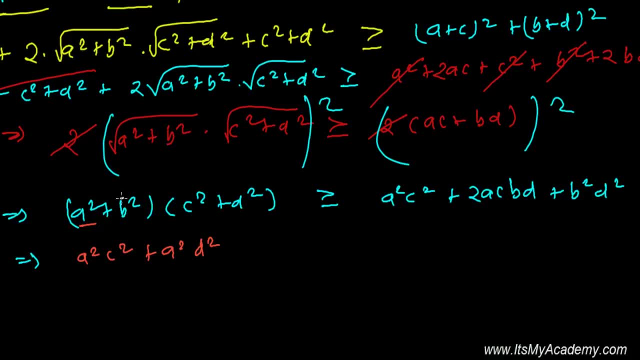 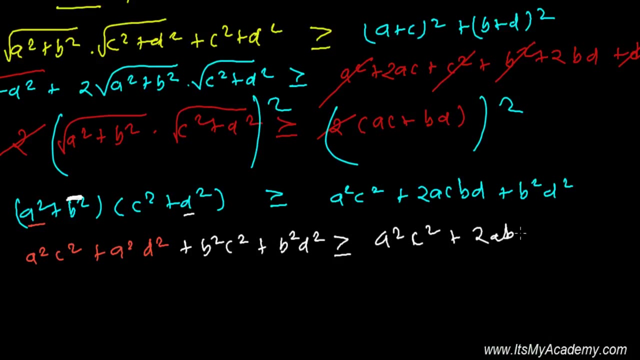 And now again, this b, b will multiply c square, so it will be b square, c square, and b will be b square, so it will be b square. b square is less than or equal to, again the whole thing. a square c square, 2, a, b, c, d plus b square d square. okay, a square, c square. 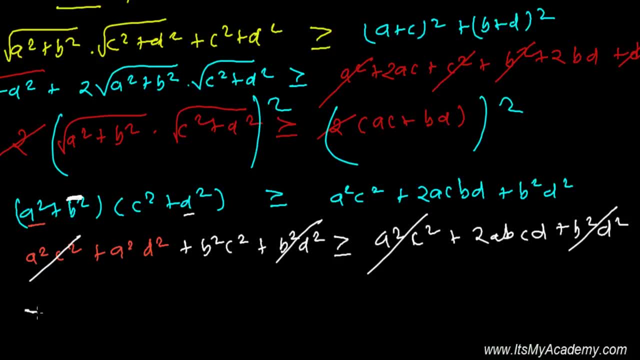 a square, c square, b square d, square, b, square d square. we can select and now see: here we have here a d whole square plus b c whole square. and here we have, uh, this plus will come this side, so it will be 2 and a, d and, uh, we can definitely do b c. all right, that is 2, a, b, c, d is greater than.